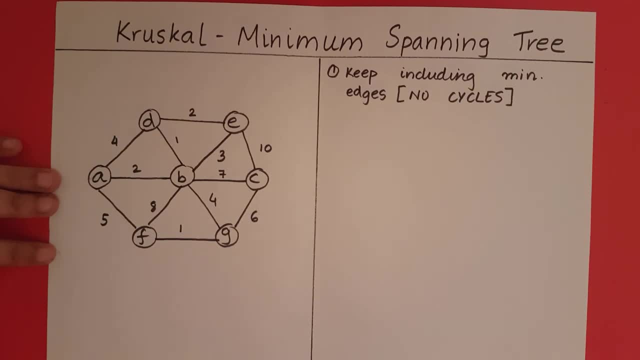 edges and we know that the subgraph is going to finally contain all the vertices. lets first draw all the vertices. so our subgraph is going to have, or our minimum spanning tree is finally going to include, all the vertices. now lets start including the edges. what are the minimum? 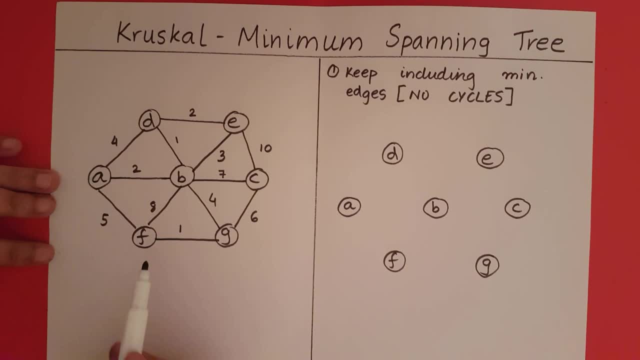 edges in this set. we have a minimum edge 1 here and a minimum edge 1 here. so first let me include this. now the minimum edge is this, so i will include that. now in this set, what is the minimum edge? we have a 2 here and a 2 here, so first i will include this, then i will include this, then i have an edge. 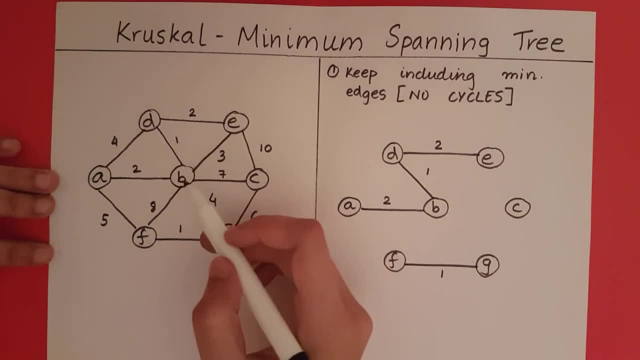 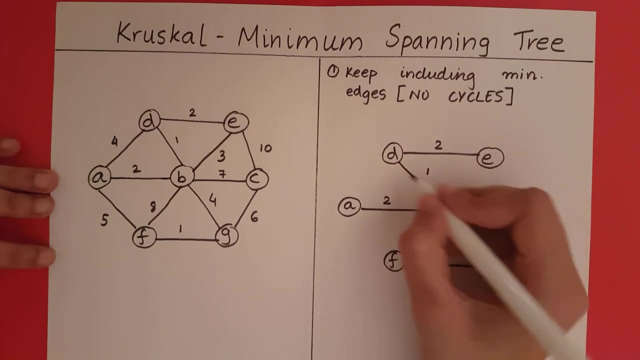 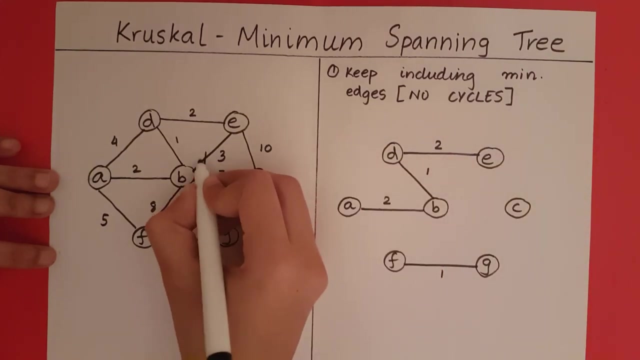 of 3, which is the next minimum edge. now can i include this edge 3? no, i cannot include 3. why can i not include 3? because when i include 3, i will be forming a cycle between b, d and e. so since it forms a cycle, i cannot include 3. now i go to 4. i have two 4s here. can i include? 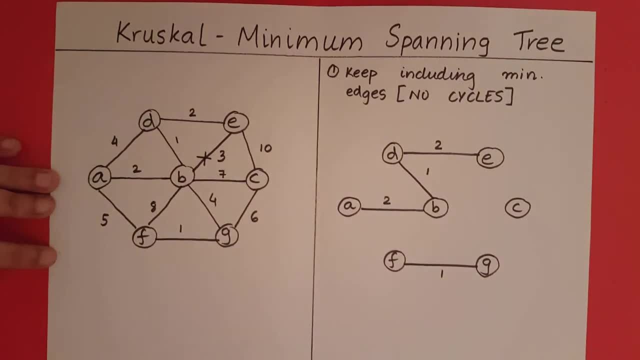 this 4? no, i cannot include that 4 because that would create a cycle between d, b and a. can i include this 4? yes, because that does not form a cycle. now i go to 5. can i include this 5? no, because that forms a cycle. what is the next largest? we have 6 or the next? 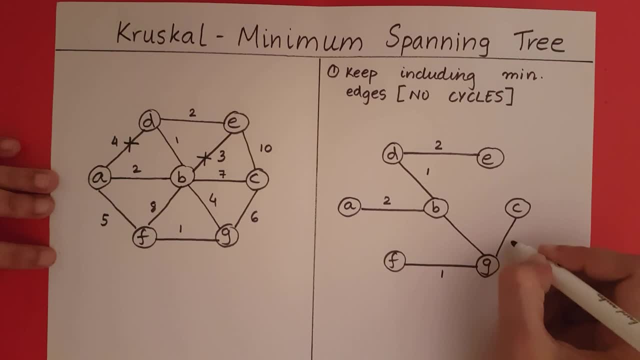 smallest. we have 6. yes, we can include 6. so now we have connected all the vertices in our minimum spanning tree. now we can stop. so what is the weight for this minimum spanning tree? we have 6 plus 4 plus 2 plus 2 plus 1.